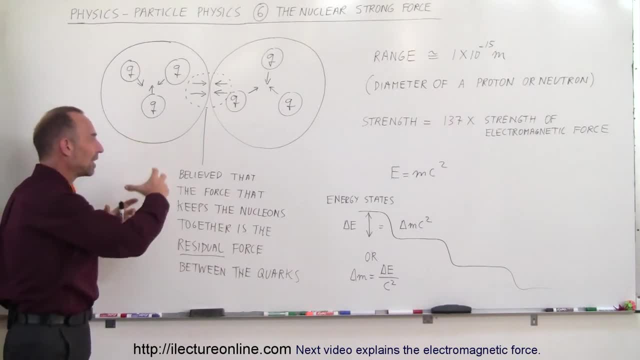 relationship between how the strong force interacts with the quarks and how the nuclear strong force to give a particle like a neutron and a proton mass. Of course there's other interactions with the boson effect and we'll the Higgs boson effect and we'll talk about that later. But what you have 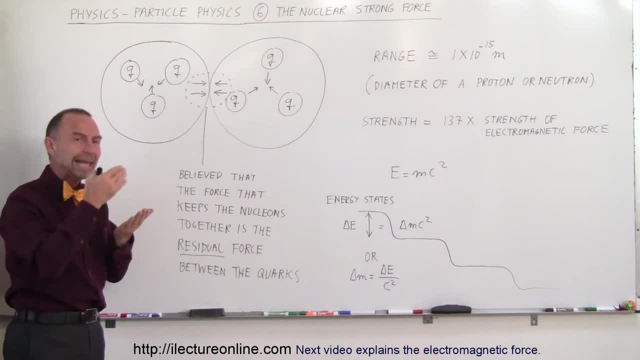 to realize is that there's a strange interaction between energy created by the, what we call the energy state of the forces keeping those quarks together, and the mass of these particles. What's also believed is that the primary function of the strong force is to keep the quarks together. 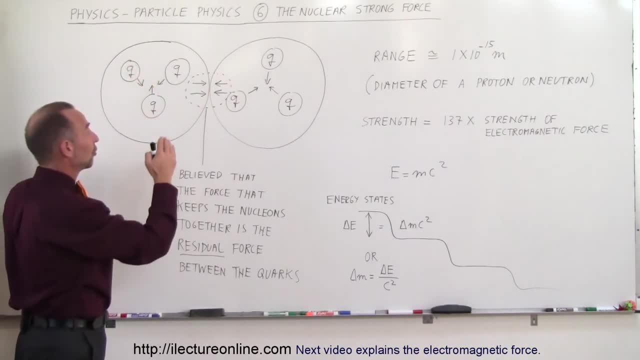 to form hadrons and to form. there's particles that have three quarks and there's particles that have two quarks- and we'll get into that detail later as well. But it's the strong force that keeps those quarks together and the fact that nucleons such as protons and neutrons are attracted to one. 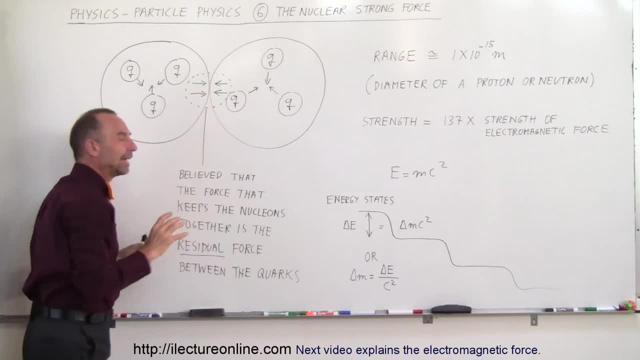 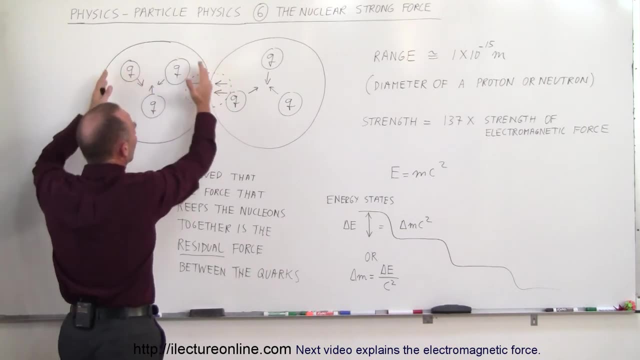 another by by the effect of the strong force is that there is a residual effect between a spillover of that force that goes beyond the boundary of the proton-neutron. that causes the protons and neutrons to attract each other, And that's what we're going to talk about in the next video. 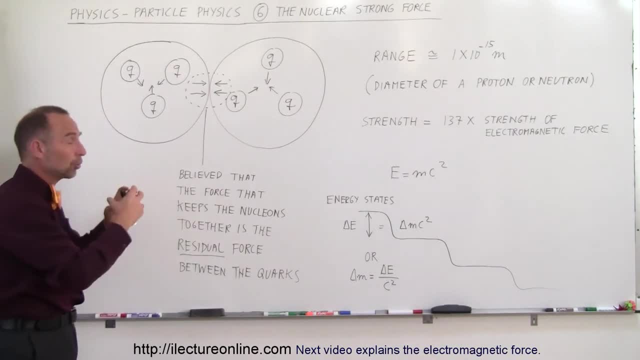 So why do protons and neutrons be attracted to each other? So protons are attracted to protons and protons are attracted to neutrons by this residual effect of the nuclear strong force keeping the quarks together. So that's why the nuclear strong force doesn't care if the 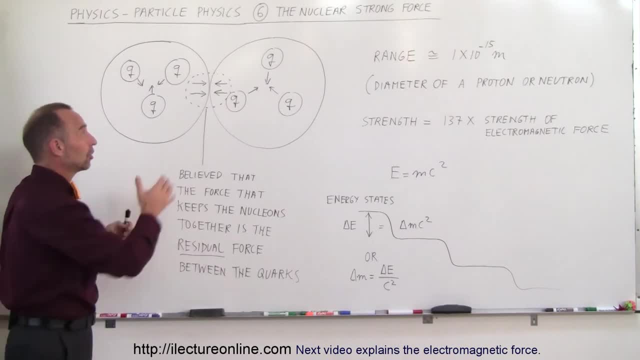 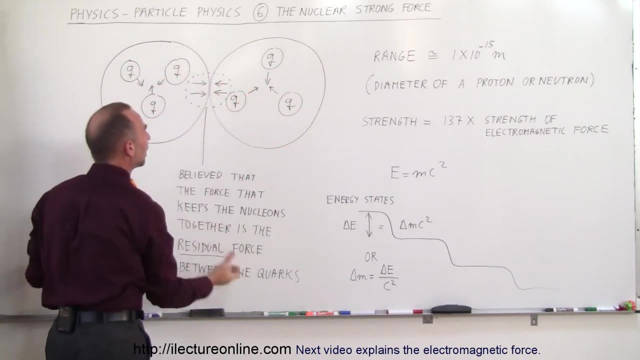 particles are charged, positive or negative, or if the particles are not charged at all, The nuclear strong force is simply there keeping the nucleons together, forming the nuclei of an atom. And so you can see that, since the primary function is there- to keep the quarks, 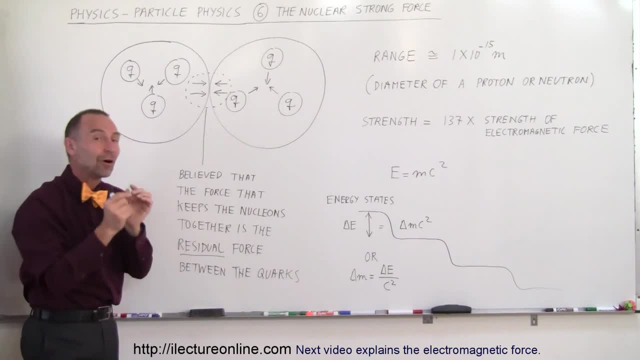 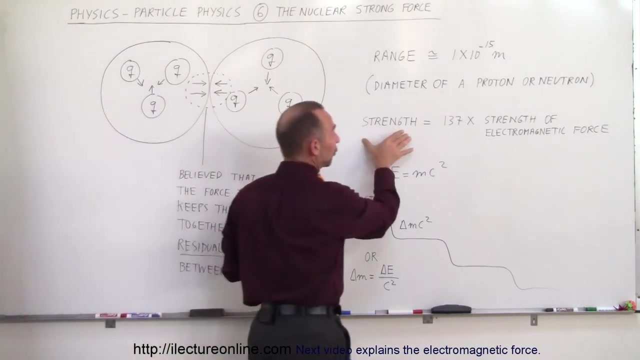 the amount of force keeping the nucleons together is far less than the force keeping the quarks together, But still it's sufficient to overcome the repulsive forces of the nucleons if they're both positively charged, And that is because the strength of the strong force is so much larger than the strength of the electromagnetic force. 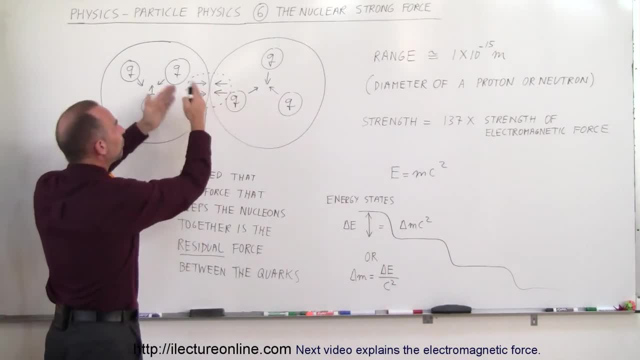 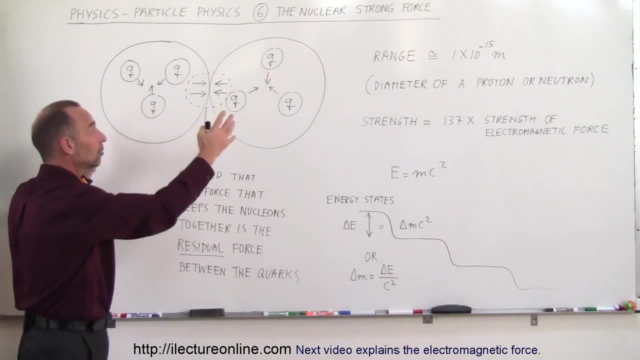 that even the spillover force between the nucleons is sufficient to keep the nuclei together, Except for the very big ones, the ones that have dozens, if not hundreds of nucleons, like for the very heavy atoms, those nuclei, they have so much repulsive force built up between them, within them, I should say. 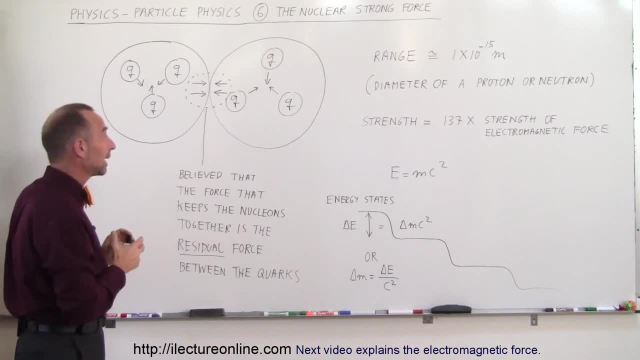 because of all these protons that are in those large nuclei that the nucleus strong force can barely keep them together. And if the nucleus gets too big for the very heavy particles, the ones that are no longer on the periodic table, the repulsive forces are just too great for the nucleus strong force to keep the nucleus together. 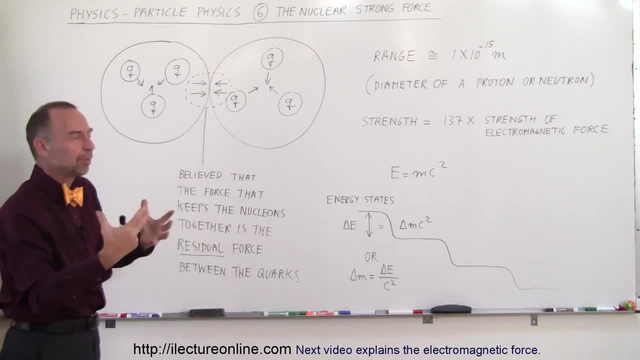 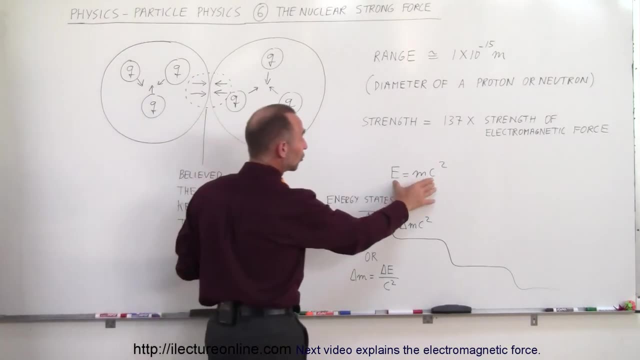 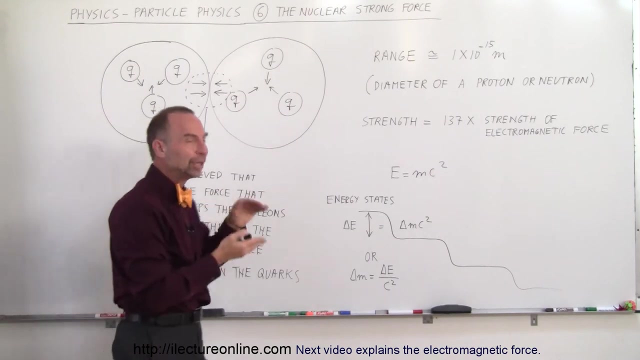 And those nuclei. those nuclei tend to be radio-activists, we call them. they tend to split apart into smaller, smaller nuclei. Another interesting way to look at it is to go back to the equation equals mc squared, is to realize that how the quarks are bound together causes these nucleons to be in a certain energy state. 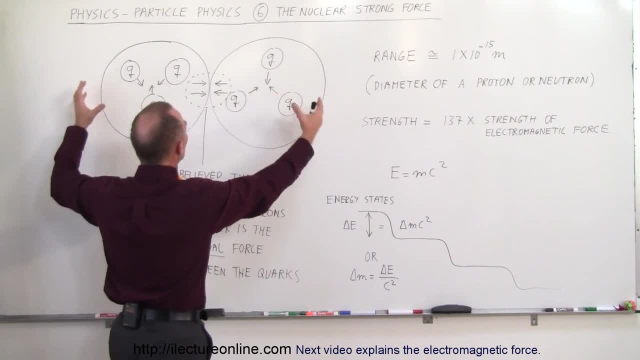 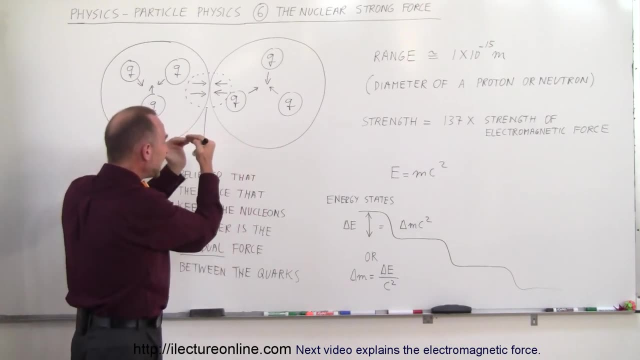 And if you then take two nucleons together, so for example a proton and a proton, or a neutron and a neutron, or a proton and a neutron, it doesn't matter if you bring them together. they are in a lower energy state, And that lower energy state means that they give up a certain amount of mass. 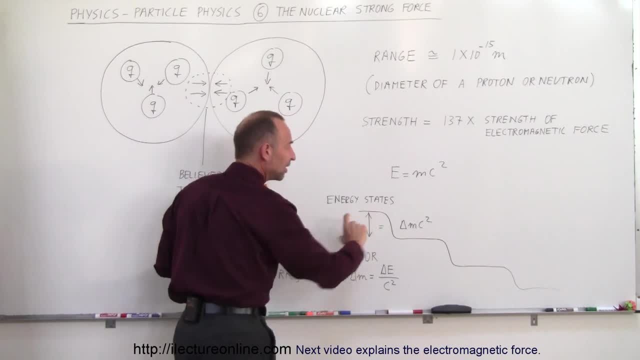 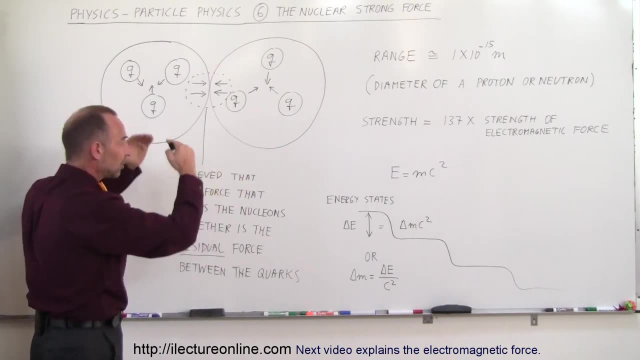 And the amount of mass that they give up is proportional to the difference in the energy state by being in, by being attracted to each other by the nucleus strong force. So when they come together they go into a different energy state, a lower energy state, and release that additional mass. 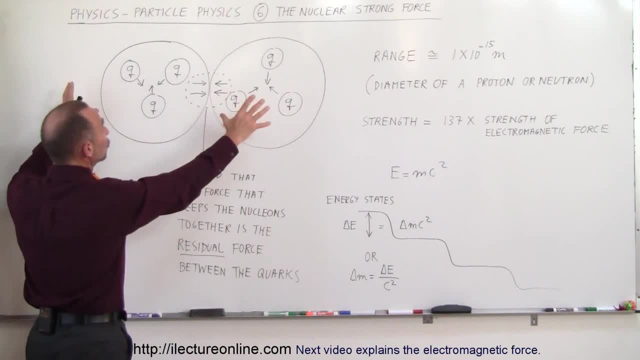 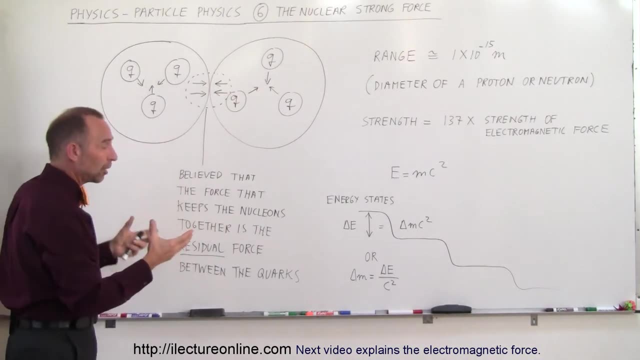 So what's interesting is that if you, let's say, you have two neutrons and you measure the mass of a neutron by itself, and then you bring them together, or if you take a neutron or a proton, you measure the mass separately. 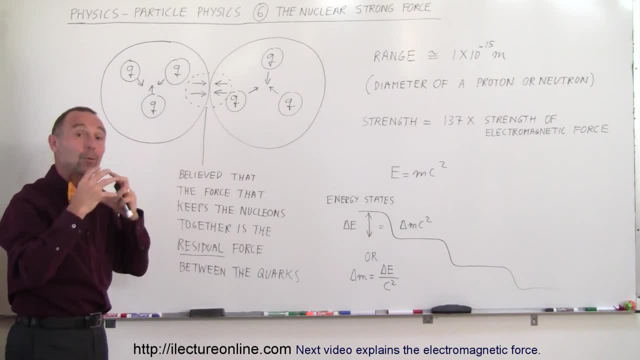 and then you bring them together. together they weigh less or they have a smaller mass than when you were to measure them individually. And that's because by bringing them together to the nucleus strong force, they lower the energy state, and a lower energy state means you release some mass. 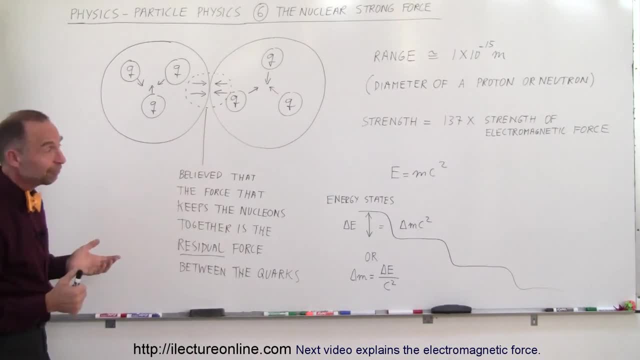 and they then end up having less mass, Very ingenious structure, and we'll learn more about that later in some other videos as well, But at least now you have an idea of what the nucleus strong is. The nucleus strong is their force. Therefore, it's used to keep quarks together. 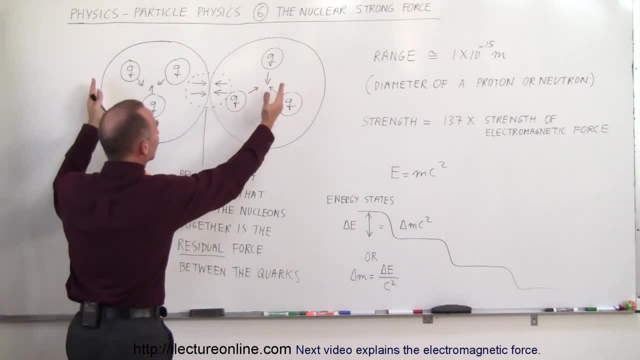 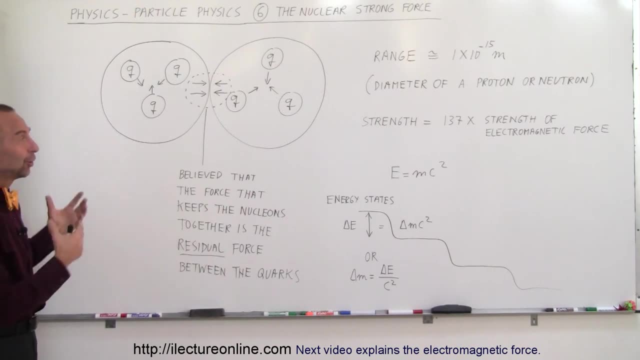 and the overspill, like the residual effect of this nucleus strong force, allows the nucleons of the nucleus of an atom to stay together as well, And without that there would be no universe, there would be no nuclei, there would be no quarks held together.